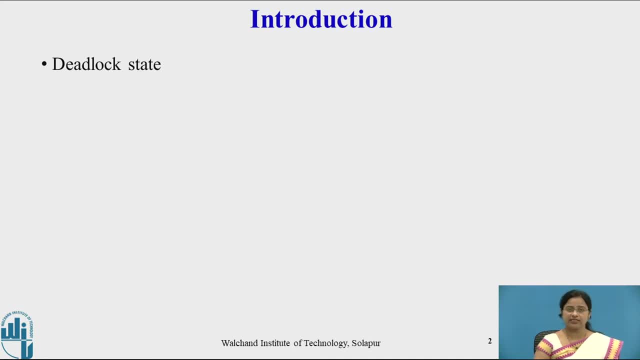 we already studied: when process enters in deadlock state, then system is in deadlock state. So in deadlock state, processes never finish their execution and all system resources are tied up. Okay, So as system resources are tied up and processes are in wasting state, they prevents all deadlock. So in deadlock state, processes never finish their execution and all system 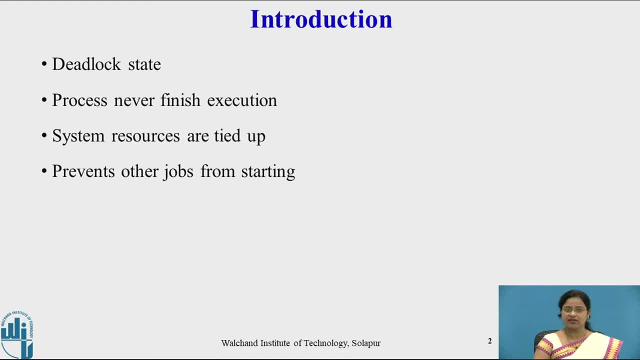 other jobs from starting, So no fruitful task is performed. So how this situation occurs in the system, So in deadlock characterization we are going to study four necessary conditions which are necessary for deadlock to occur in the system. So deadlock can arise if four conditions hold. 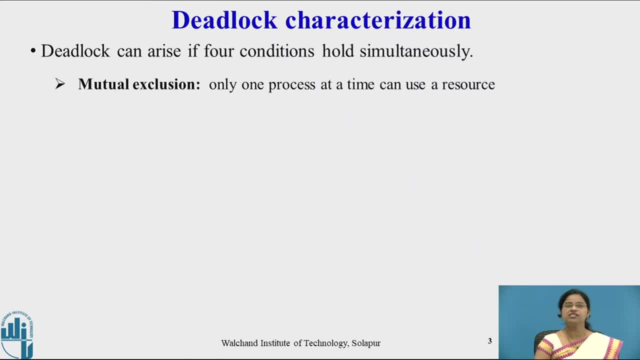 simultaneously in the system. First is mutual exclusion. In this case, only one process at a time can use a resource. If the resource is already used by that process, then next process will enter in waiting state. That process will not use that resource. So here as we can see, if process P1 is 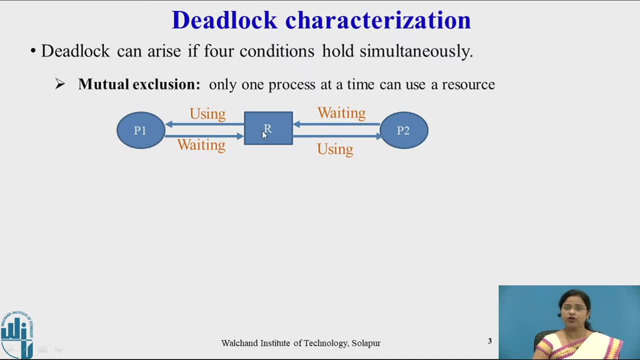 using resource R, then P2 must wait for that resource. But if P2 is using the resource R, then P1 must wait for the resource. This situation is called as a mutual exclusion. Then next is hold and wait, A process holding at least one resource is waiting to acquire additional resource held by other. 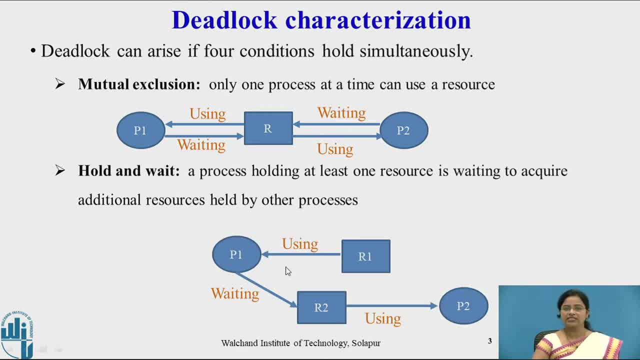 process Means process is already holding one resource. For example, here P1 is already holding R1 and it is waiting for R2, which is already used by P2.. Okay, So this is what the process is: holding one resource and waiting for another resource. that is hold and wait. The next is mutual exclusion. 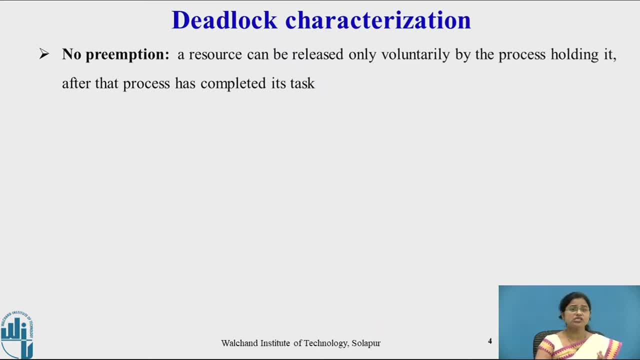 No preemption. Now, no preemption means here a resource can be released only voluntarily by process, holding it after that process has completed its task. Means the resource once it is allocated to the process, then that resource is never deallocated till process complete its execution, That resource. 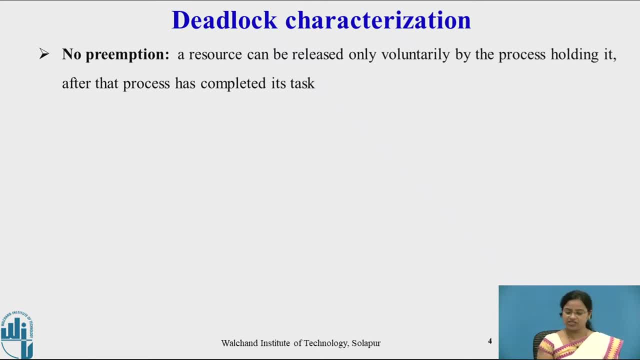 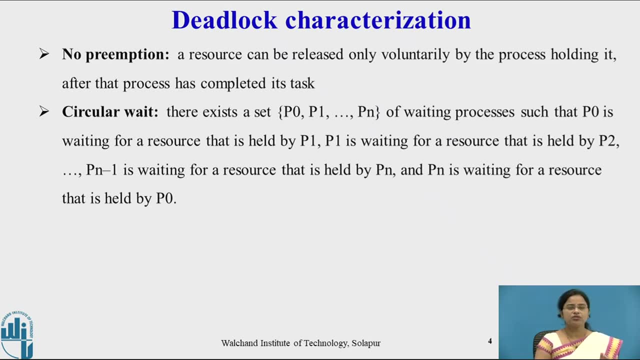 will be with that process till it completes its execution. It is never preempted. Next condition is circular wait. So in circular wait, Suppose there exist process P0 to Pn and these processes are waiting like that: P0 is waiting for P1, P1 is waiting for P2, P2 waiting for P3, P4 waiting for P5 and again P5 is waiting. 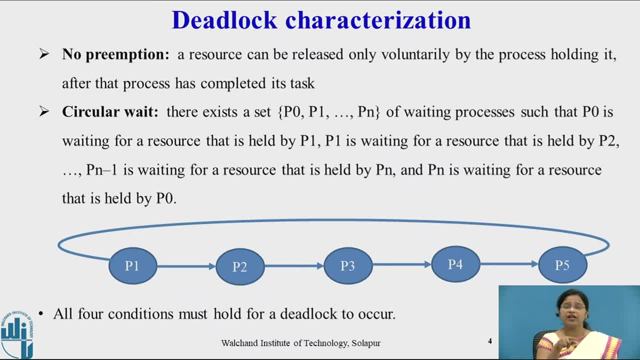 for P1.. So this situation is called as a circular wait, Means here: one process, previous process, is waiting for next process, then next process, then next process and the last process is again waiting for the first process, is called as a circular wait. so when these all four conditions are exist simultaneously in the 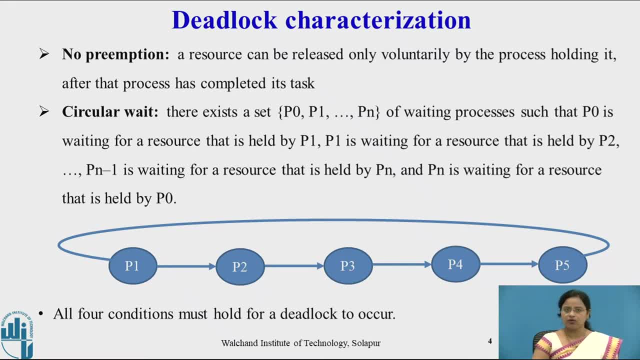 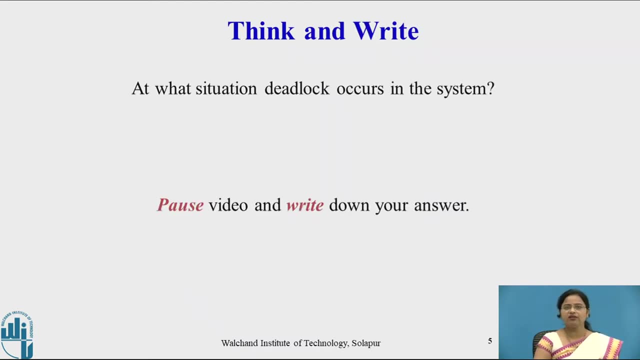 system. then we can say that deadlock occur okay, that four conditions are: mutual exclusion, hold and wait, no preemption and circular wait. if all these four conditions are there, then deadlock occur in the system. so just pause the video and write what, in what situation, deadlock occurs in. 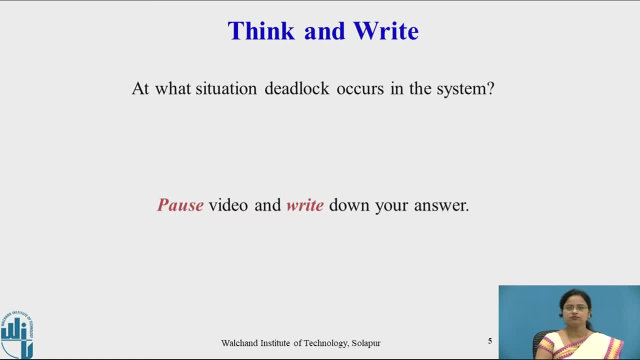 the system. so deadlock occur in the system whenever all four conditions hold simultaneously in the system. now the next concept we are going to study is resource allocation graph: how resource allocation graph plays an important role for the detection of the deadlock. now, what is this resource allocation graph? it is a system resource allocation graph which is nothing but a 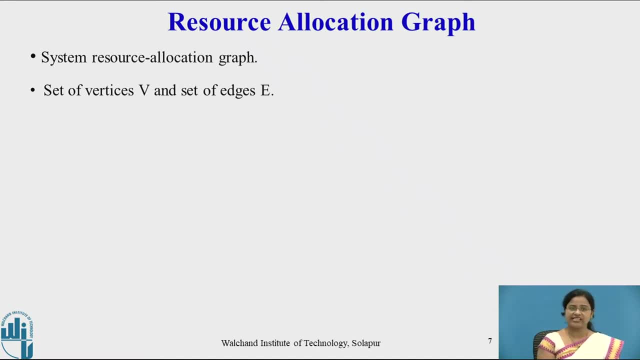 deadlock set which contains set of vertices v and set of edges. it is a directed graph with set of vertices and set of edges. set of vertices are divided into two parts. first is number of processes- p1 to pn- and number of resources- r1 to rm. so processes and resources are denoted and as a vertices and 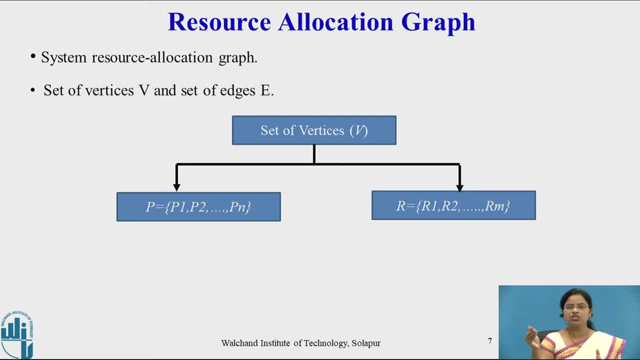 request made by process to the resource and allocation of the resource to process is indicated as a edges. so the directed edge from process to resource is called as a request edge and the directed edge from resource to process is called as a assignment edge. so we will see the notations. 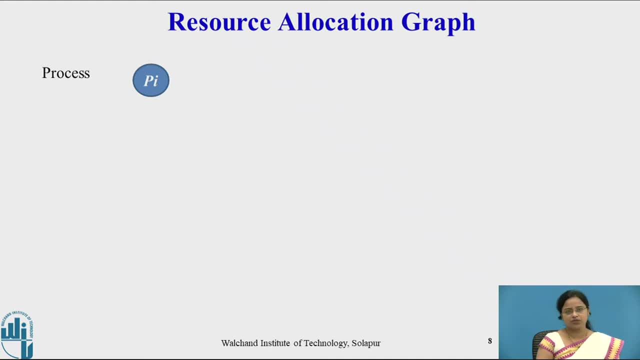 which are used in resource allocation graph. first is process. process is denoted as a circle with its number. then resources are indicated by a rectangular block, block with instances as a dot or a dot and a square. now here i use square. in your book we have a dot for instances of the resource. now here, 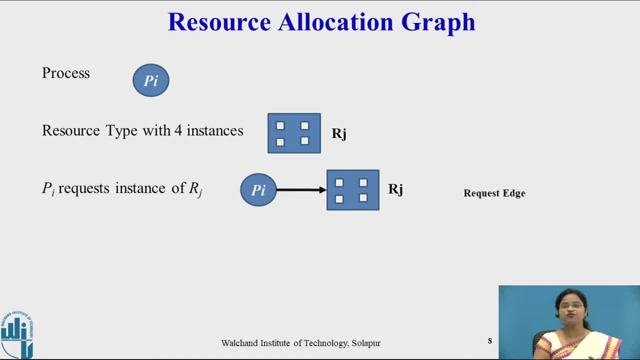 process. when process pi request for resource rj, then that request edge is shown. whenever the process, one of the instance of the resource, is allocated to the process, then it is shown as a assignment edge. now consider a resource allocation graph. here we have three processes and four processes are allocated to the process and the other three processes are allocated to the. 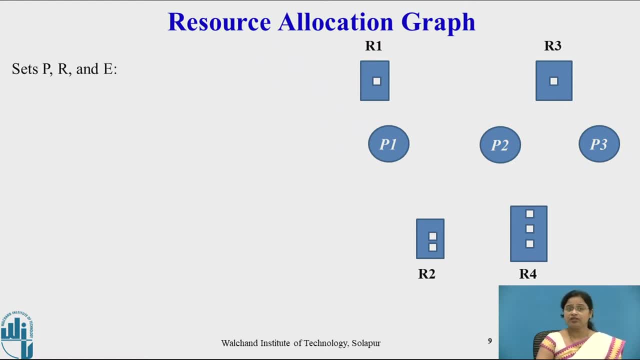 resources. okay, so we have a set of sets of process resource and edges. now set p will contain p1, p2, p3, r will contain r1, r2, r3, r4. and now the set of edges from p1 to r1, r1 to p2, r3 to p3, r2 to p2, r2 to p1. 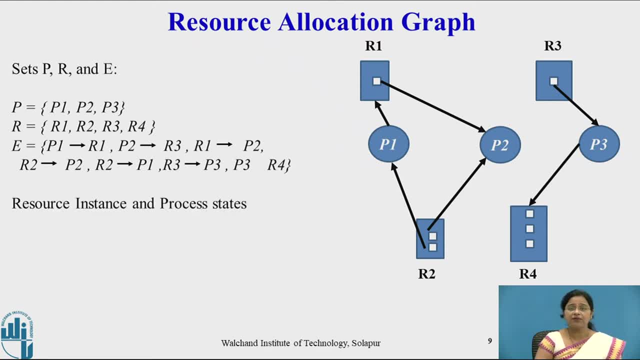 and then we have r, p3 to r4 and p2 to r3. so these are the set of edges. so this shows the resource instances and the process states. okay with request edge and assignment edge. now here, this is nothing but the assignment edge, which is from r1 to p2 and p2 to r3. 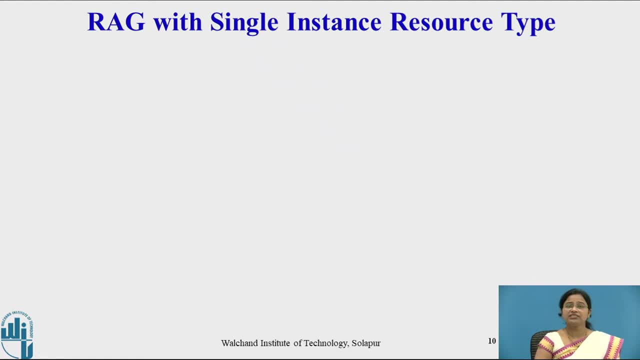 is nothing but the request edge. so this is how the resource allocation graph can be drawn, based on number of processes, number of resources and how the request and allocation is given to the process. now, in this case, we have a set of resources and we have a set of resources and we have a set of. 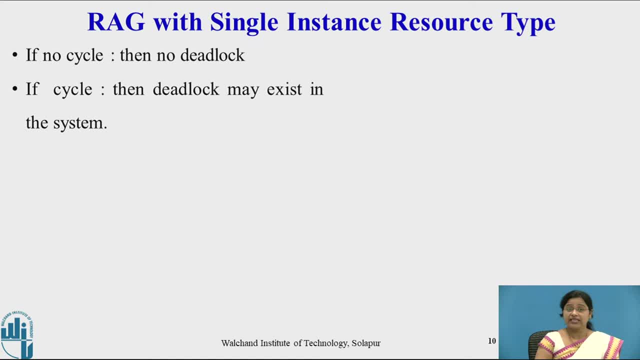 the process called resource allocation graph and because if the process is given here, we have to obtain the process. we have toabano provide idnd in the job. so even if rocket is being developed for every object, whether it will beрыt treatment or streaming or robust application, however, all day long generating the village is not enough. 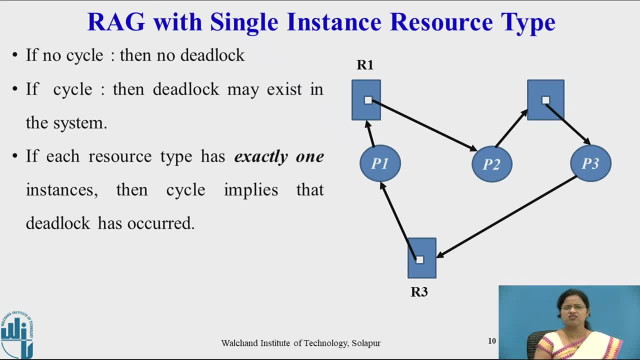 if it will be Michael gyle creating the Valley Control Management System. we have to calculate the defendant. the jurisdiction is a limit. all right, we have to to a function. So enter to dot. we simply call it data order table, so we can decorate it as we want and 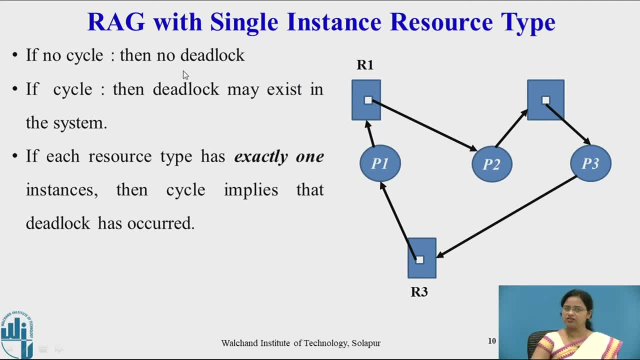 So, as shown here, if there is no cycle, then there is no deadlock. If cycle exist, then deadlock may exist in the system. If each resource type has exactly one instance, then cycle implies that deadlock has occurred into the system. If we have only one instance, then this we can say that there is a cycle from P1 to P2,. 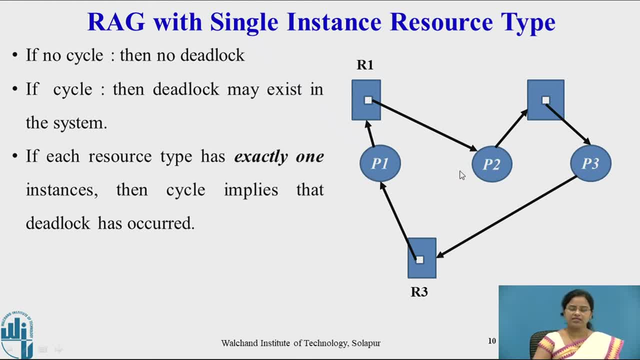 P2 to P3, again P3 to P1.. So this may says that deadlock may occur in the system, or deadlock has occurred. Now we will see that how this, for single instance, the deadlock cycle, is a necessary and sufficient condition for existence of the deadlock. 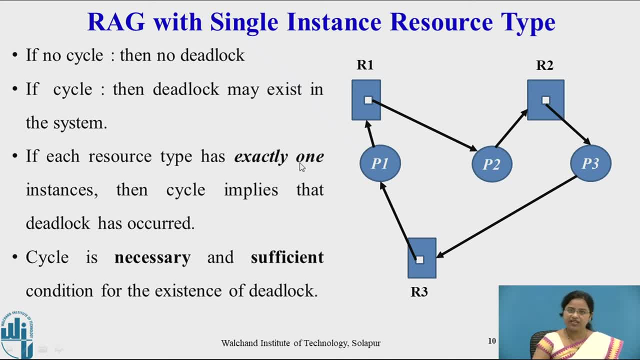 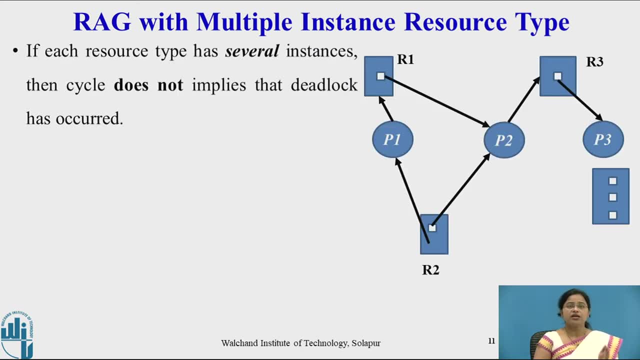 So if we have a single instance, then we can say that if there is a cycle, deadlock surely occurred in the system. Now, if we have multiple instances of the resource type, multiple instances of the resource type, if cycle exist, then it does not imply that deadlock has occurred. 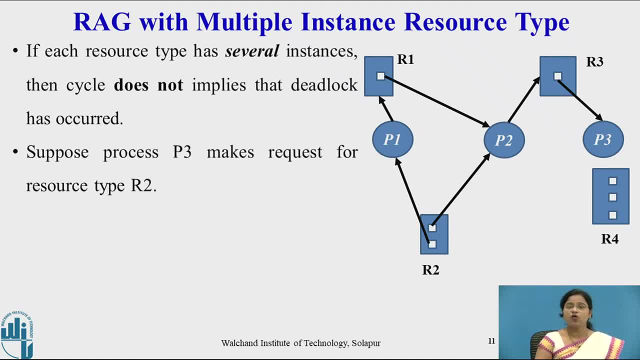 So, as shown here, we have 3 processes and we have 4 resources, and this is how the request and assignment age are given. Now, this is the current situation. Now suppose process P3 make request for an instance of resource type R2, then we will. 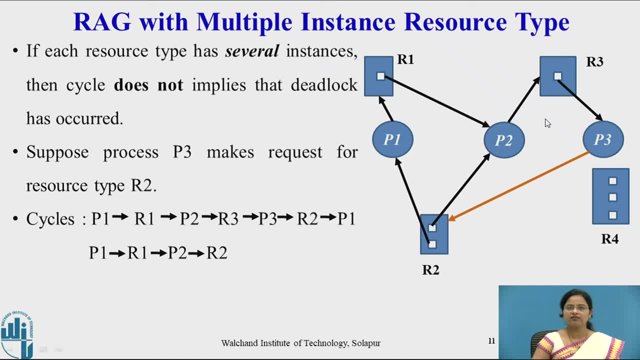 have the cycles like this: P1 to R1, P2 to R3, R3 to P3, P3 to R2 and again from R2 to P1 or R2 to P2.. So this: there may exist a cycle. 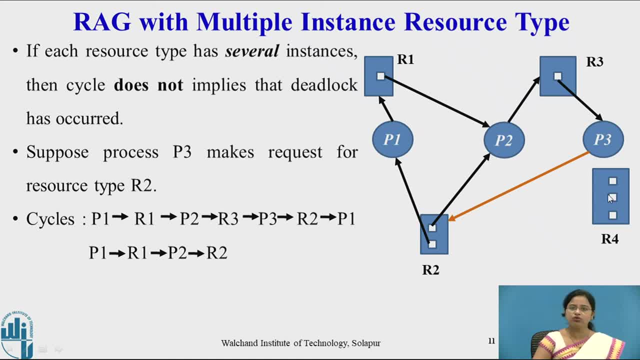 So this is the current situation. There may exist 2 cycles, from P1 to P3 to P1, or from P2 to P3 and again P3 to P2. But here, whenever this cycle exist, then we can say that this P1, P2, P3 are in deadlock. 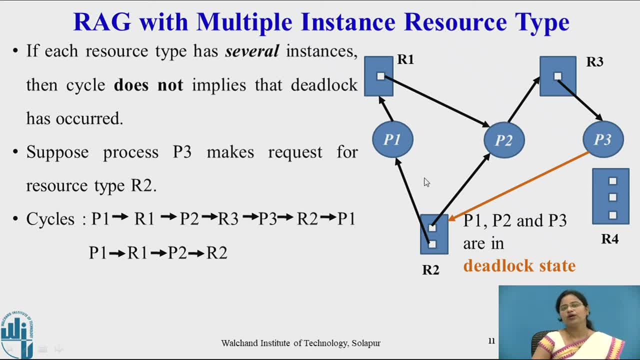 state because both of the instance of R2 are one is given to P2 and one is given to P1, and P3 will enter in waiting state. So cycle exist. so this is the deadlock state, But for whenever we have a multiple instance. 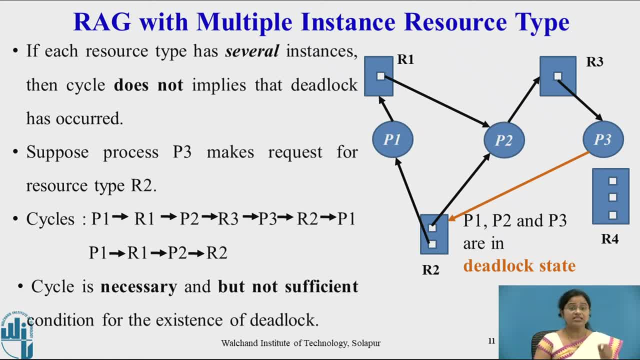 Then we can say that cycle is necessary but it is not sufficient condition for existence of the deadlock. For single instance cycle is necessary and sufficient condition for the existence of the deadlock. Now how this is necessary, but not sufficient condition for existence of a deadlock that.